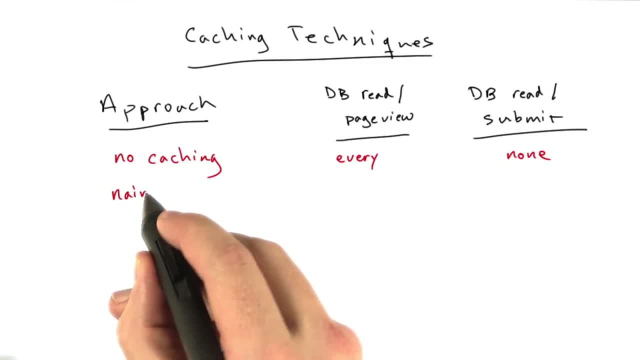 Then we did this kind of what I would describe as the naive caching approach, which was basically have the basic cache, If the cache is empty, do the DB read and if it's not, return the result, And we'll add a third column on the edge here called bugs. 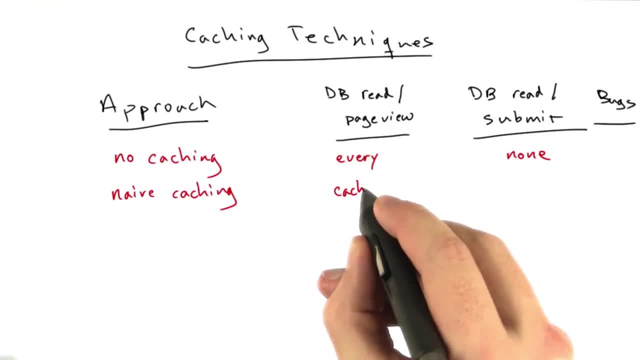 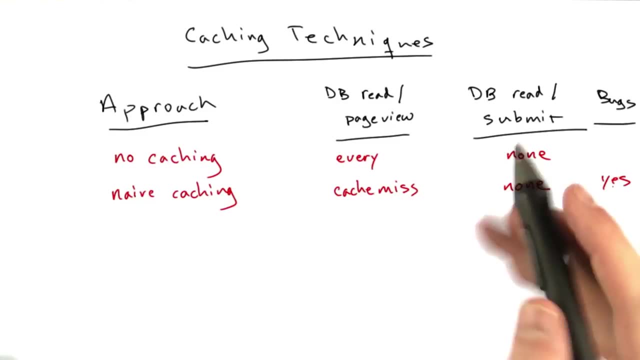 So the naive caching only does a DB read on a cache miss and doesn't do any reading on a submit and is full of bugs, or at least has one bug where the front page would become out of date, that the front page would become stale. 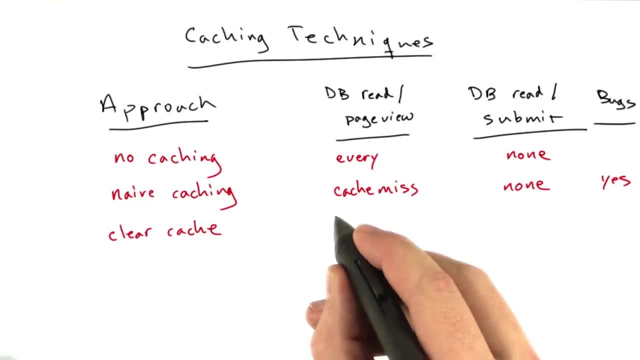 So then we started clearing the cache. This has the same property of doing a DB read on a page view, no DB read on a submit and no bugs. Then we improved to the kind of the refreshing part- refreshing of the cache- And so this means we're no longer doing any DB reads on page views, or very rarely. 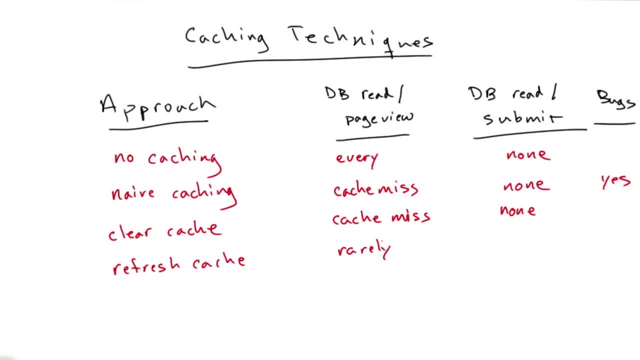 basically only the first time our app turns on and the cache is empty and that first page view. Every other page view after that is cached, which is a really nice property to have, And we're doing one DB read per submission and it works. 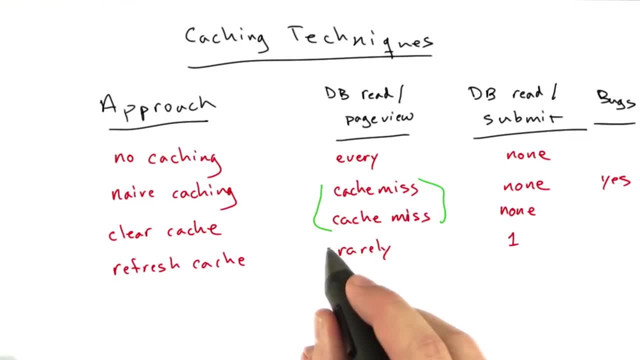 Now the difference between these two and this one is the notion that a page view doesn't hit the database hardly ever, And that's a really nice property to have. You should always be striving to have the situation where a normal unlogged in basic viewer of your website doesn't touch the database. 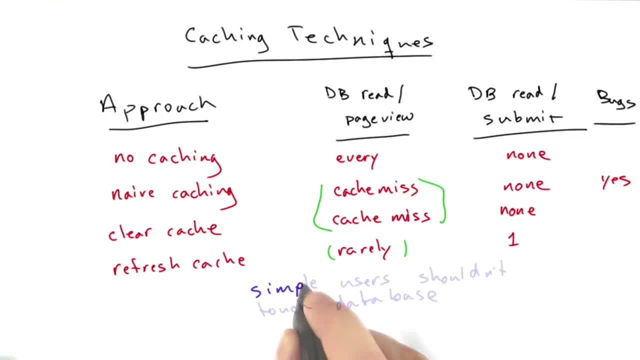 And I'm going to kind of condense that down to the notion that simple users shouldn't touch the database. Basically, they're just lurkers, They're just reading, They're not changing the site, so they shouldn't be touching the database. 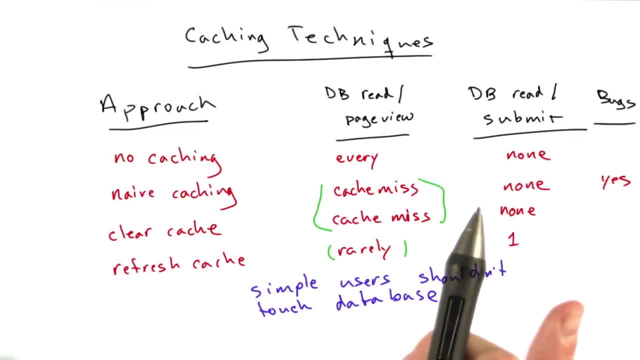 Everything should be cached and ready to go for them. That makes the user experience better, because the request will be faster and it keeps your load down, because you can add many, many of those users And because they're just bouncing off the cache. 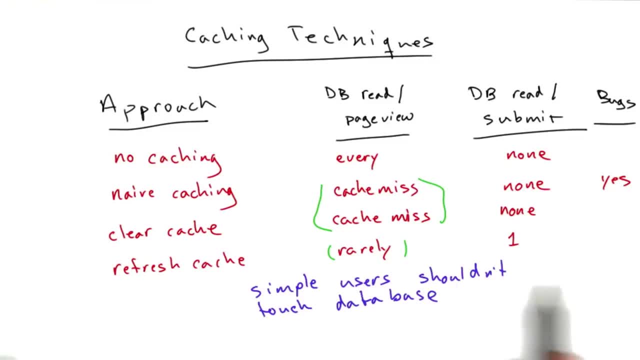 you don't have to do very much work to serve them, You don't have to actually hit the database. Now there's a fourth approach that we didn't implement yet, which is the most aggressive of all of these, And I'm going to kind of refer to this as distinct from refreshing the cache. 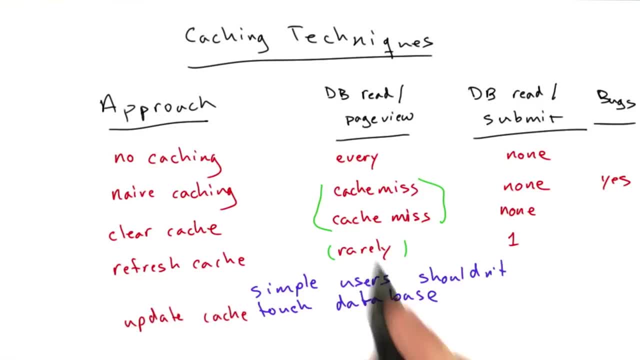 I'm going to call it updating the cache And I'll talk about this approach in just a sec- And we can get to the state where on a page view, on a simple page view, we do zero DB reads ever, And this is slightly better than rarely. 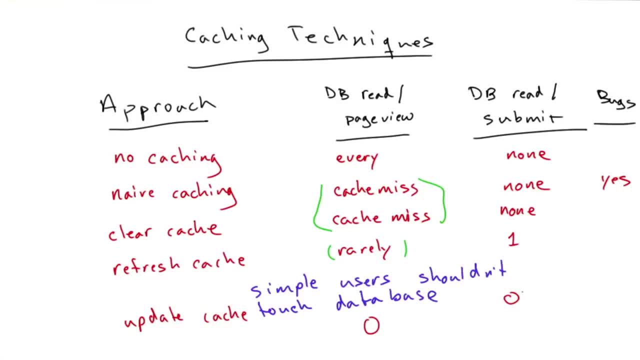 And we don't do any database reads on submission either, And it works. This is a really nice property to have. Now, of course, we still do our database write. You notice we haven't been optimizing writes at all, because you've got to store the submission at some point. 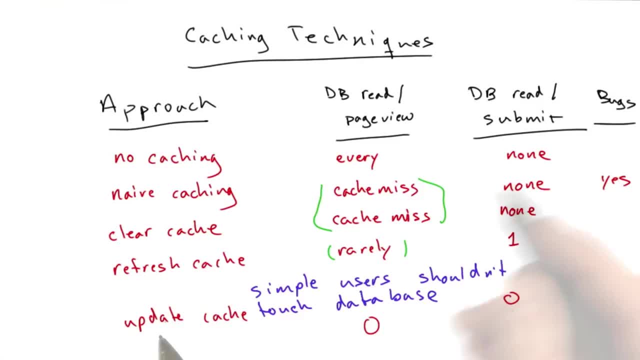 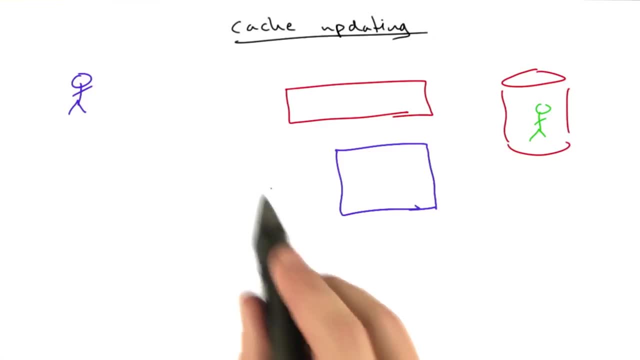 But you can cut down on the database reads, lower them to both zero by keeping your cache completely up to date, And I'll show you how we might do that right now. Okay, we're going to look at this picture one more time here. 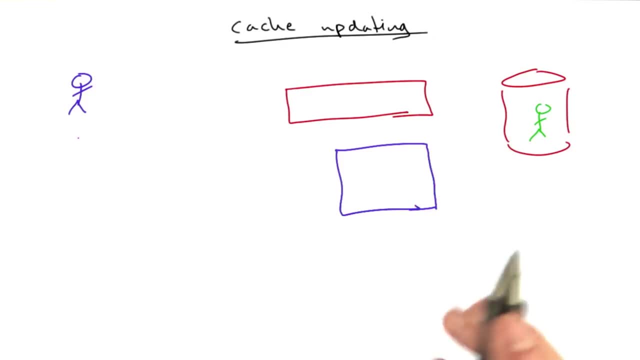 We know all the pieces now. We know the user, the ASCII channel, the database and our cache. We're going to talk about a new situation here, So let's pretend our cache is already warm. It's got some pictures in there. 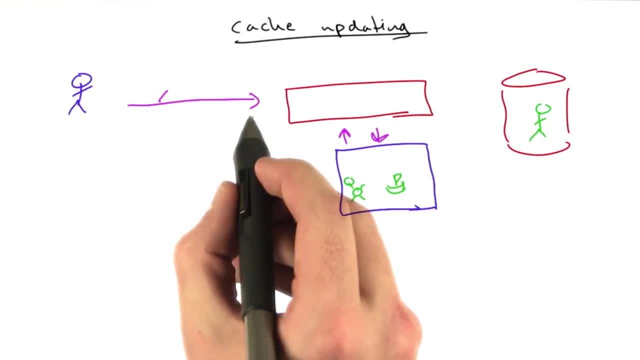 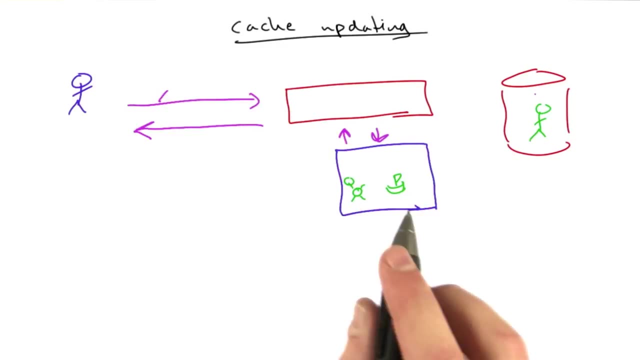 And we're hitting the front page, which hits our cache, which returns the result that we send back to the user. Nothing too complex. there We're not hitting the database because we're only doing reads. Now what happens is when we do a database write. 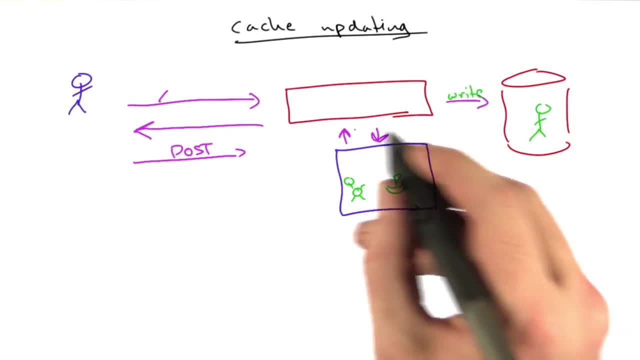 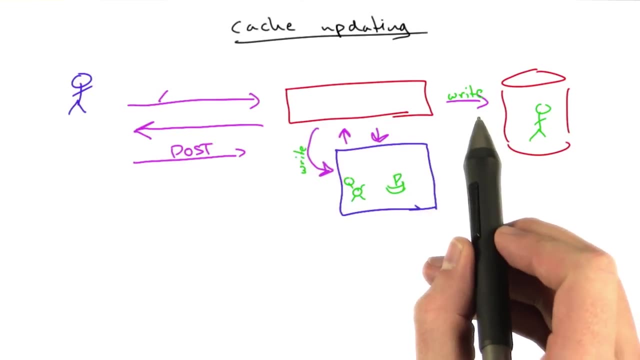 we're going to send that write to the database. We're simultaneously going to send that write to our cache as well, And so this gets a little bit more complex. We're going to send the write to the database And instead of immediately rereading from the database to update our cache. 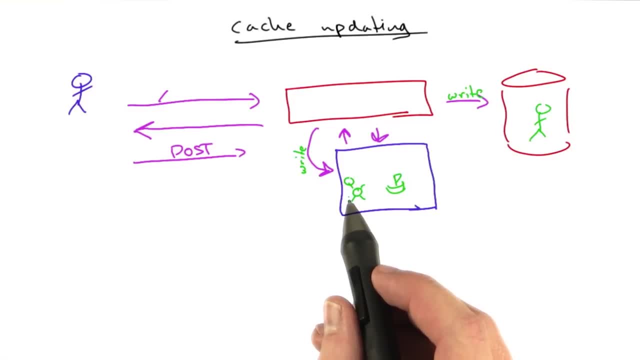 or clearing our cache. we're just going to update the cache. We're going to say, okay, this affects the front page, so let's find that front page cache, insert our new piece of ASCII art into the cache And then, from then on, that follow-up request, that redirect. 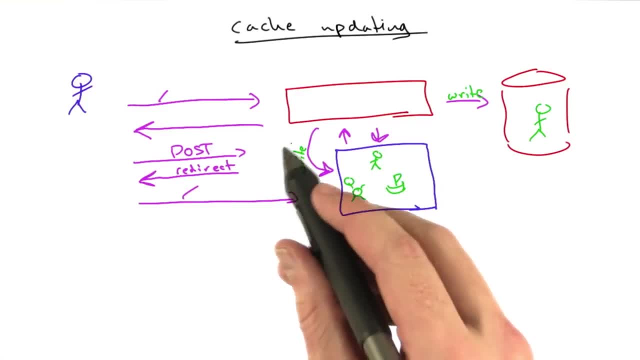 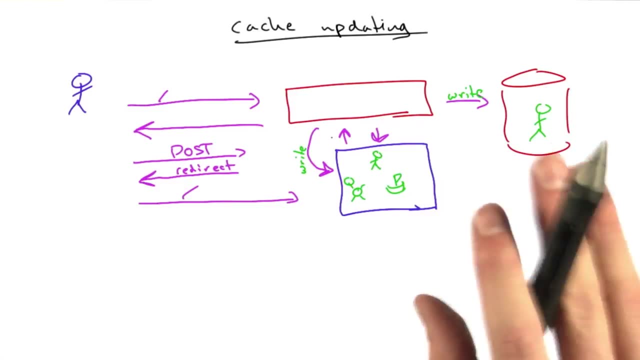 that follow-up request to slash is basically going to bounce right off the cache again, And so we never did. We never did a database read during this whole process. We're just writing only. The only time we would do a database read is when we start up the app for the first time. 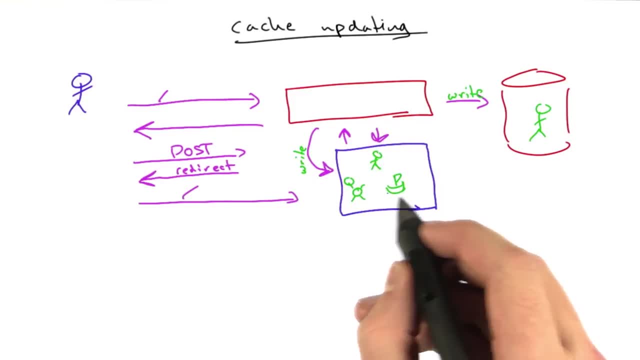 and do that first request, or maybe we have a program that does that for us, so no user ever does a database read, And this is actually how we do things on Reddit. now Every listing you can look at is stored in its own cache.